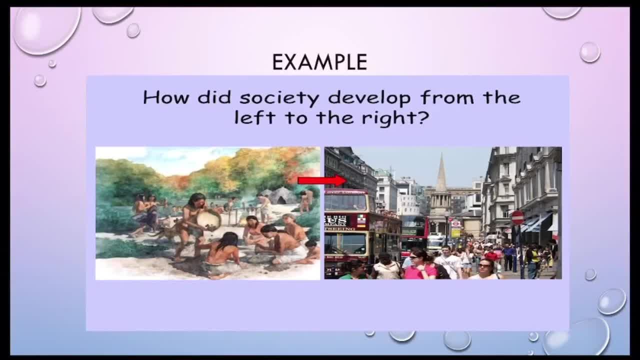 Welcome to the Veronica or WI ret CBS. You can see how different people's clothes are versus how withor the clothes on the people on the right, which is basically how we dress today. You can see how the people are basically living off the land in the left picture- OMG. 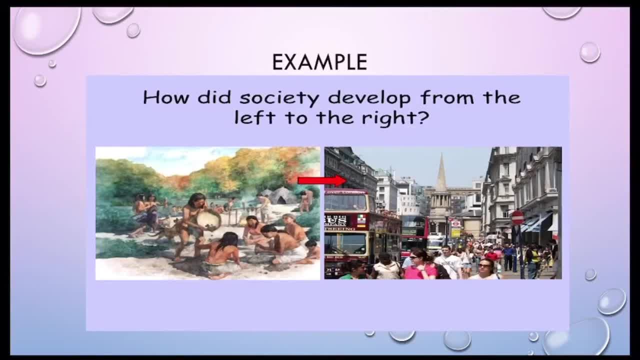 rocks to build things, how they have made a fire in the back. you can look at their homes in the back as well. look like they're made out of sticks and tree branches and things of that nature, and you can see the women over there. they're carrying different things versus the picture on the right. 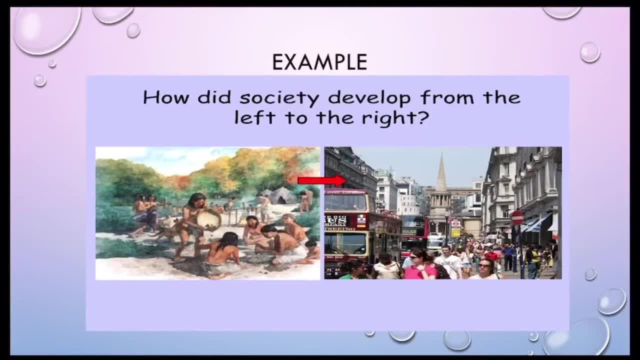 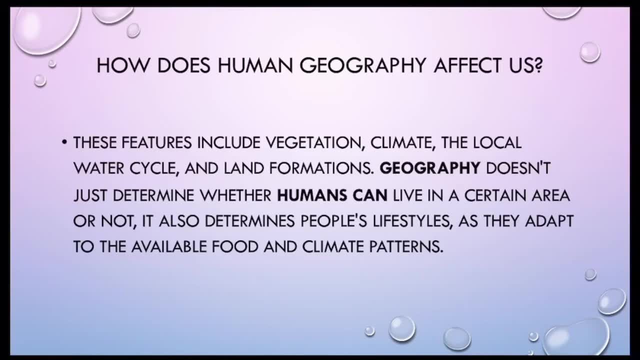 where people are just walking around, probably shopping. we see buses, we see large buildings made out of brick and stone and different things. so now we just go to the store to get all the things that we used to have to work for in the picture on the left. all right, so how does human? 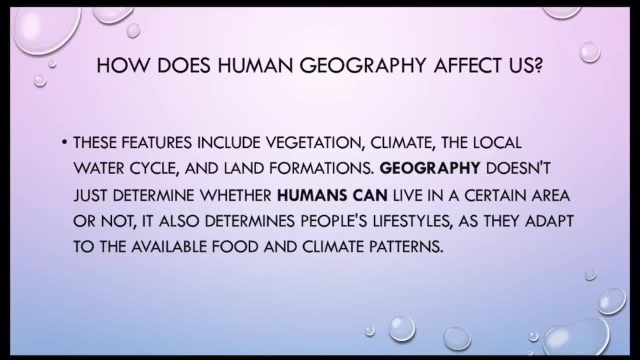 geography affect us. okay, so the features that affect us are vegetation where we live, climate where we live, our local water cycle and land formations. geography doesn't just determine whether humans can live in a certain area or not, it's all. it also determines our lifestyle and how. 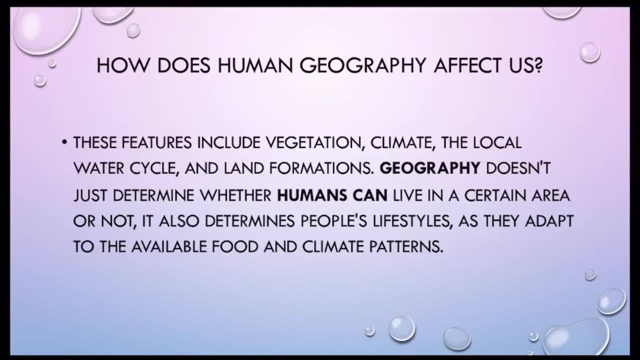 we adapt to the available flue, food and available climate patterns. so what that? what that means is wherever you live. basically that means you're going to have to adapt to where you live and how you live, and it just really is going to basically just tell us what type of lifestyles we're going to have. we want to build. 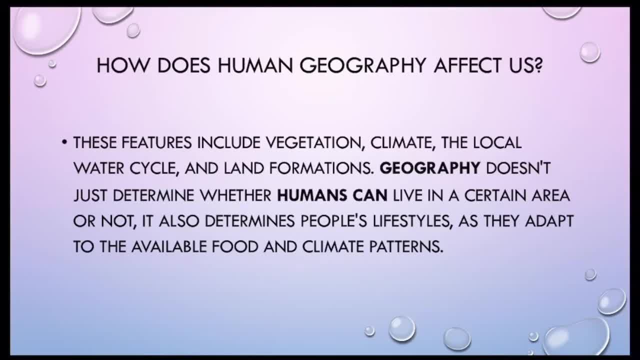 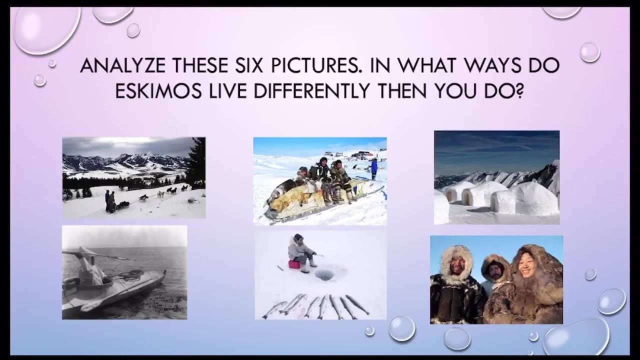 a society around those things that we have no control over, which is vegetation, the climate, local water cycles. how far do we have to walk to get water where? where are the water cycles? uh, land formations, mountains, um. cold, um. land formations, um. okay, so i want you to go ahead and look at these six pictures. here you're going to analyze the six. 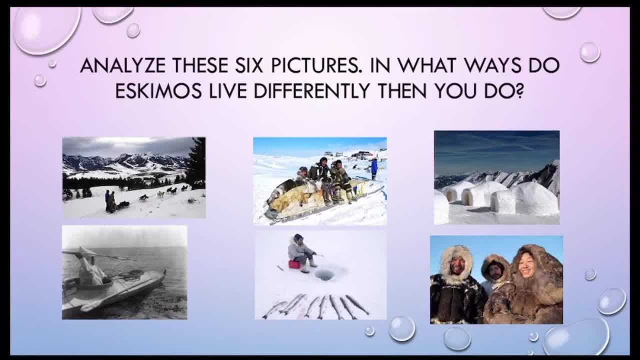 pictures and you're going to look at the eskimos and identify ways that they live differently than you do, okay, so if you take a look at the first two pictures, you will see that this is basically the way that they are transported, or their means of transportation, should i say so? they use sleds and 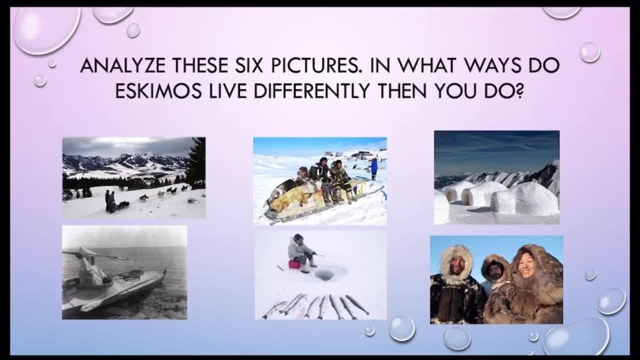 they use dogs and this is because of the climate and their land formation, so they have mountains and hills and snow and trees. so they can't just go to the mountains and they can't just go to the get in the car like we do and go where we need to go. They have to use sleds. If you look at the 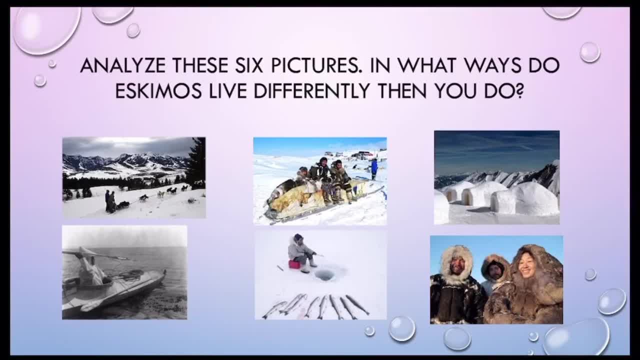 last picture, at the top, you can see that these are their homes. Well, these are their homes. They're called igloos. It's where they live, So they have to live off the land or use what is given to them. So they use the ice and they use the snow to build homes. If you look at the two, 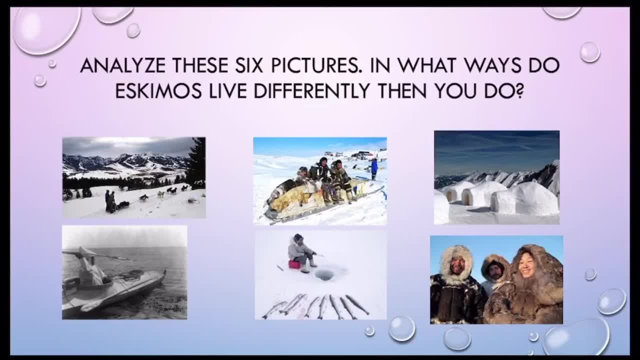 pictures. the first two pictures at the bottom row. this is how they gather their food. So they go out and they hunt. They spear fish in the first picture And the second picture he is ice fishing. They cannot just go to the local store and go grab what they need or jump on their sled and go to 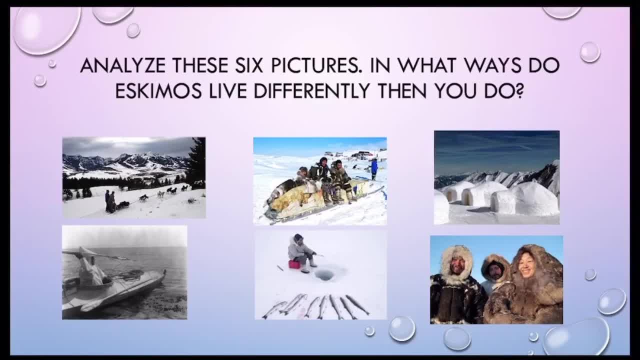 McDonald's and get them a hamburger or anything of that nature. They have to actually hunt for their food. If you look at the last picture, which you see how their clothes are different. they have to dress like this and bundle up in lots of fur in order to keep warm. That is because 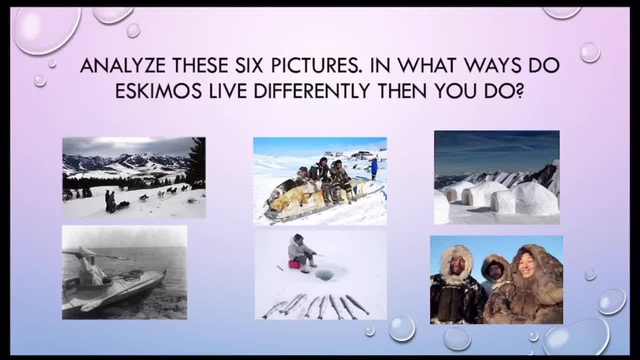 of the climate that they live in, And I'm very sure that they have gotten this fur from off of an animal that they have killed. They have used the meat to eat and use the fur to keep warm. Okay, So they live very much so differently than we do because we can just go to the store and get 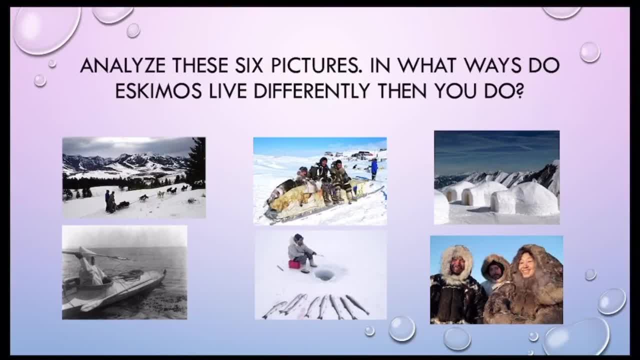 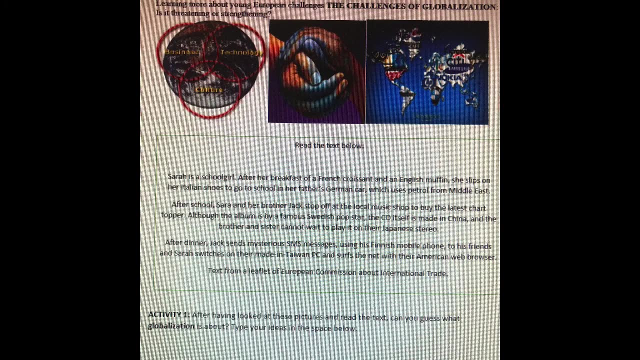 all the things that we need And we don't have to bundle up like this, because it never gets that cold here in Los Angeles. All right, So for your first activity, you're going to go back to teams. You're going to go to 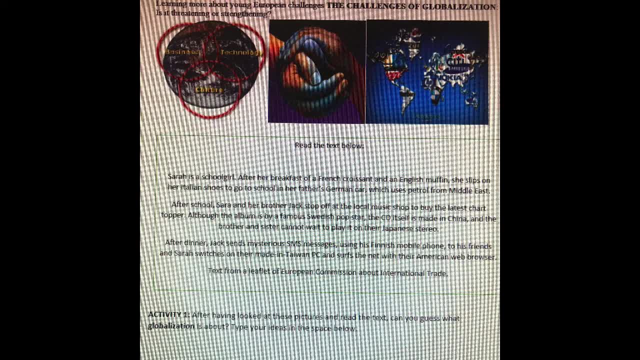 the assignment tab and this assignment is going to be there. You are going to look at those three pictures and analyze them And we're going to start to develop what globalization is. You're going to read the text in the box below. Once you do that, you're going to answer the question for activity one Once you finish that. 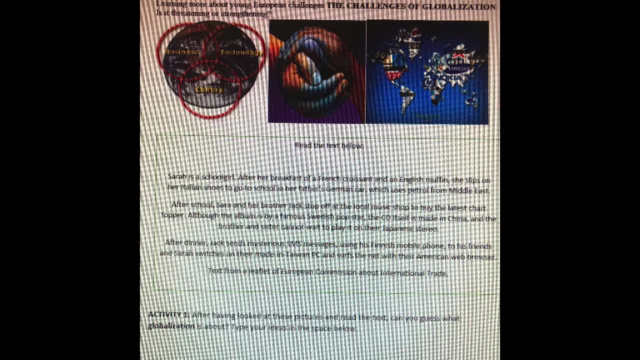 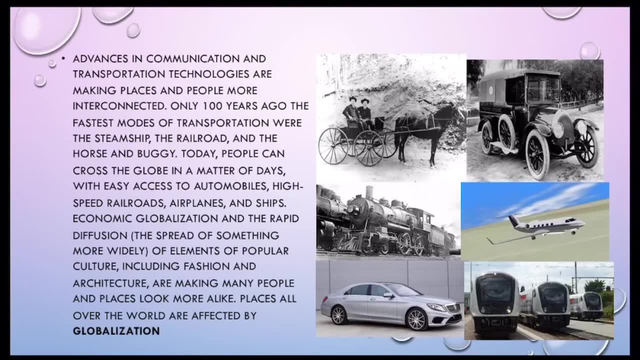 I want you to come back to this PowerPoint and begin where you left off, so we can get a good definition of what globalization actually is. Okay, And globalization is advances in communication and transportation technologies, making places and people more interconnected. Only 100 years ago, the fastest modes of transportation were the steamship. 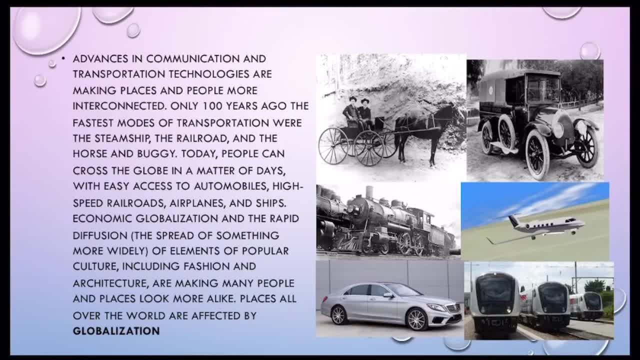 the railroad, horse and buggy. Today, people can cross the globe in a matter of days With easy access to automobiles, we have high-speed railroads, we have airplanes, we have ships. Economic globalization and the rapid diffusion, the spread of something more widely of elements, 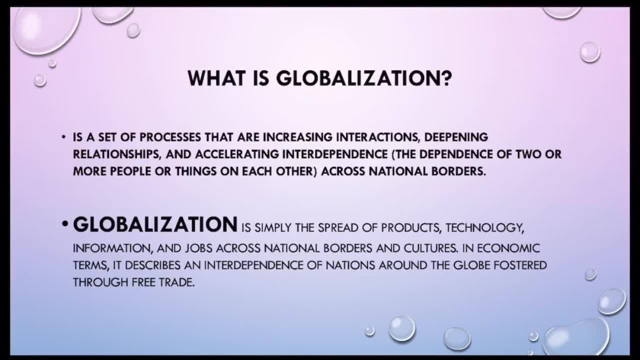 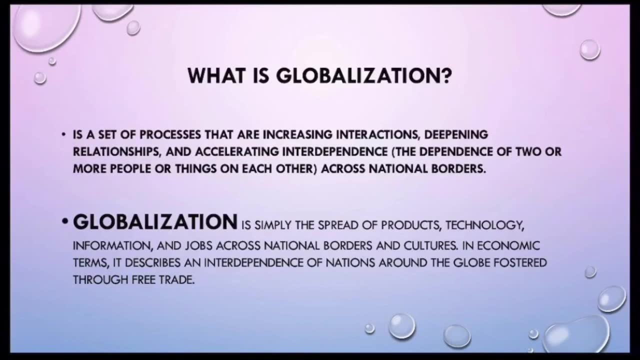 of popular culture, include fashion, architect, and they are making a way into homes everywhere. This is how globalization is affected. So what is globalization? It is a set of processes that are increasing in terms of transportation, transportation, transportation, transportation, interactions, deepening relationships and accelerating independence. That is a 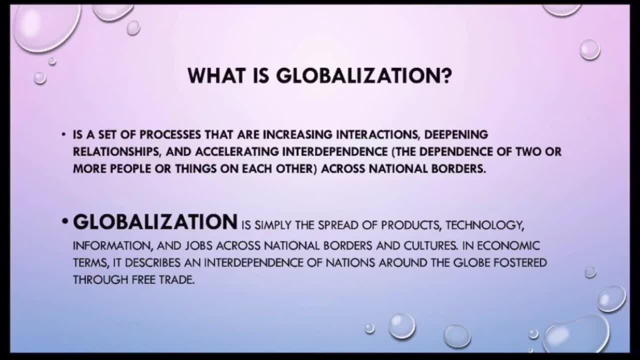 dependence on two or more people or things on each other across national borders. Globalization is simply the spread of products, technology, information and jobs across national borders and culture. In economic terms, it describes interdependence of nations across the globe, fostered through free trade. So, basically, what globalization is is how we, different nations, 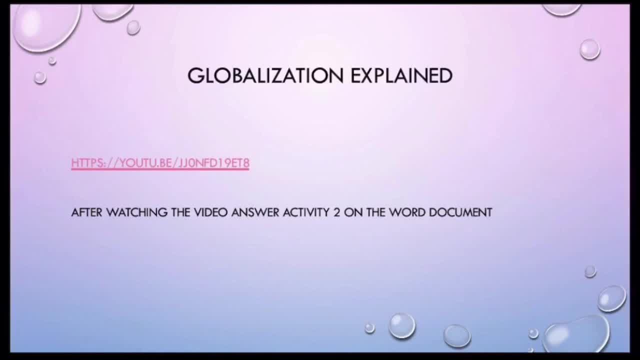 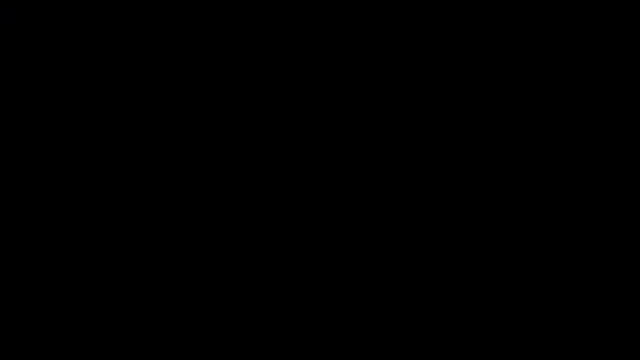 we depend on one another For different items. if you take a look at your just say, look at the tag in your shirt, it probably says made in China, or something of that nature. So we get many things from different places and this is all free trade. Okay, Now you have a second assignment activity. 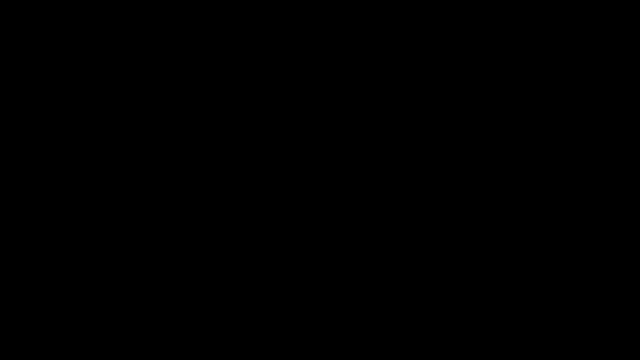 Number two: you're going to go back to the assignments tab and then you're going to watch the video on globalization. That video is going to be under the post section. It's a YouTube video. Once you watch that video, you're going to go.